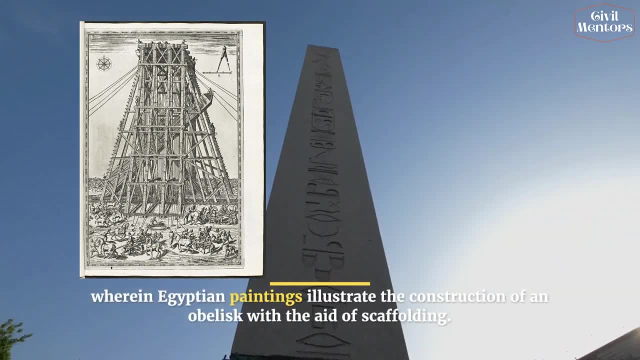 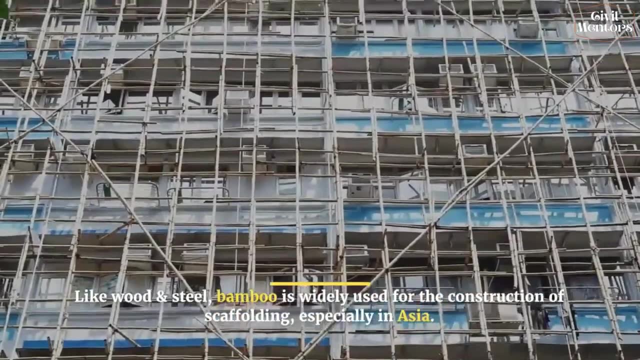 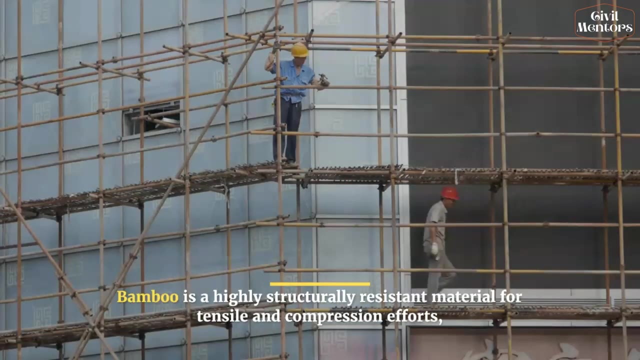 illustrate the construction of an obelisk with the aid of scaffolding. Like wood and steel, bamboo is widely used for the construction of scaffolding, especially in Asia. Bamboo is a highly structurally resistant material for tensile and compression efforts and it grows very quickly and can be harvested and used easily. 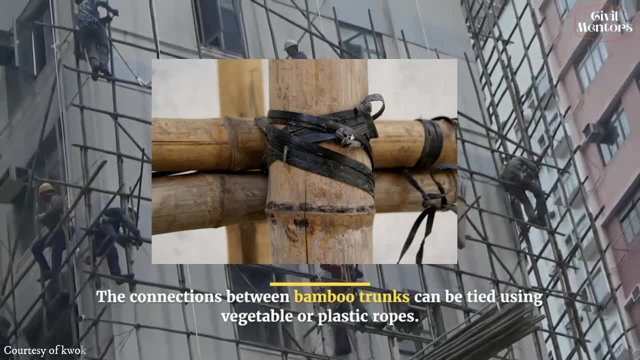 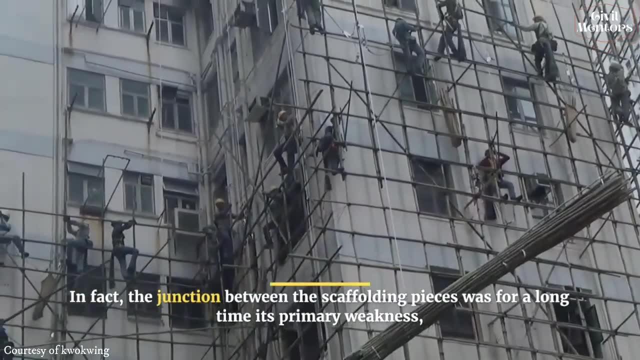 The connections between bamboo trunks can be tied using vegetable or plastic ropes. In fact, the junction between the scaffolding pieces was its primary weakness for a long time, An issue that required considerable time during assembly. An important actor in scaffolding is the use of bamboo as a support structure for construction. 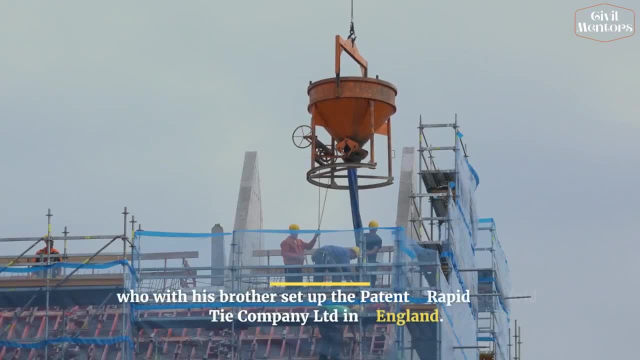 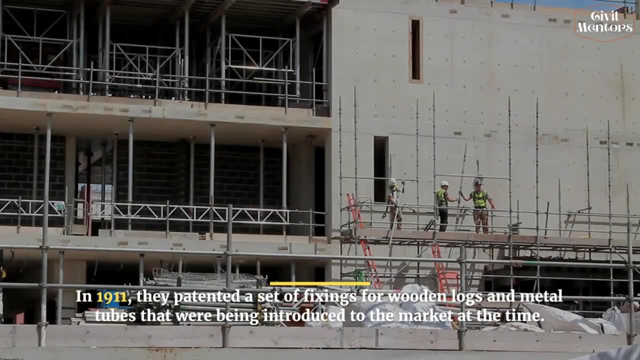 An important actor in this history was Daniel Palmer Jones, who, with his brother, set up the patent Rapid Scaffold Tie Company Limited in England In 1911, they patented a set of fixings for wooden logs and metal tubes that were being introduced to the market at the time. 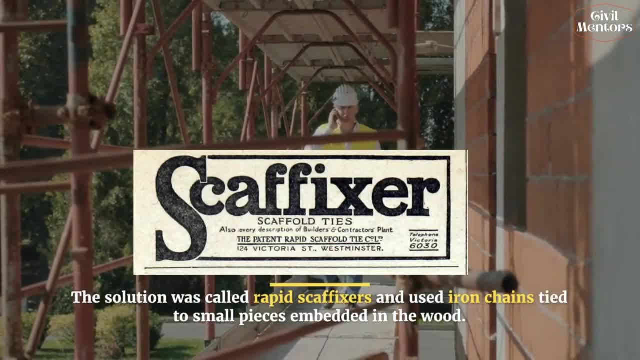 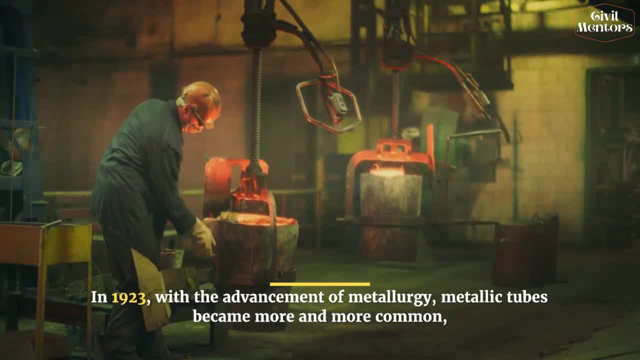 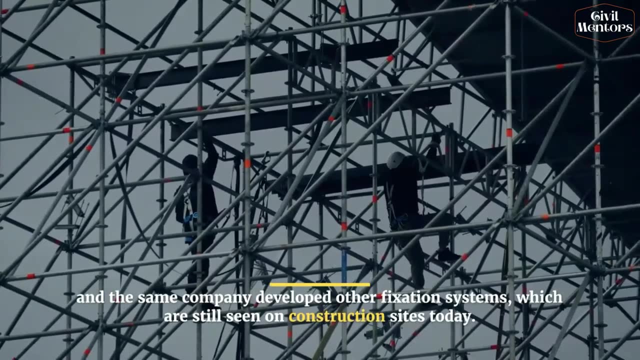 The solution was called Rapid Scaffixers and used iron chains tied to small pieces embedded in the wood. In 1923, with the advancement of metallurgy, metallic tubes became more and more common, and the same company developed other fixation systems which are still seen on. 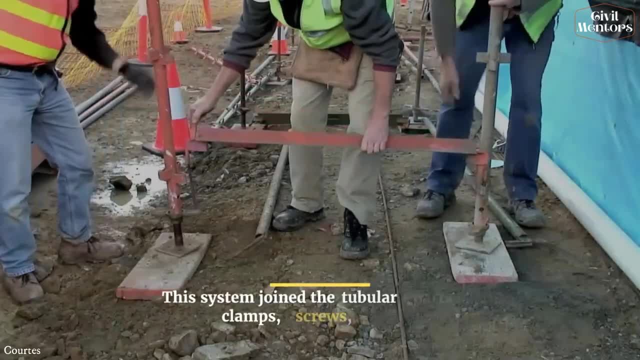 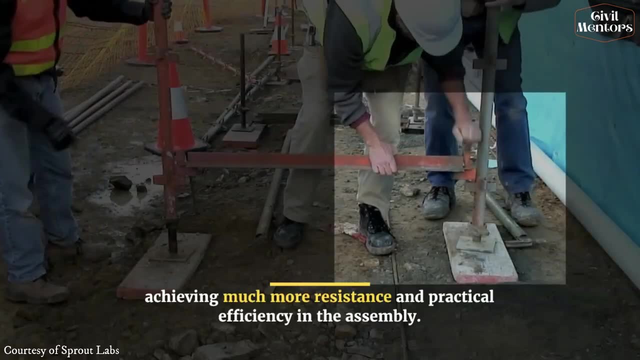 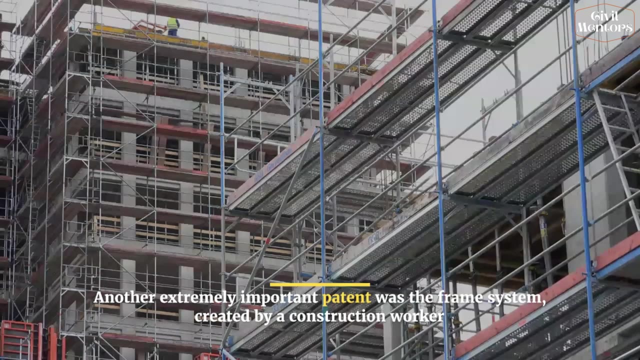 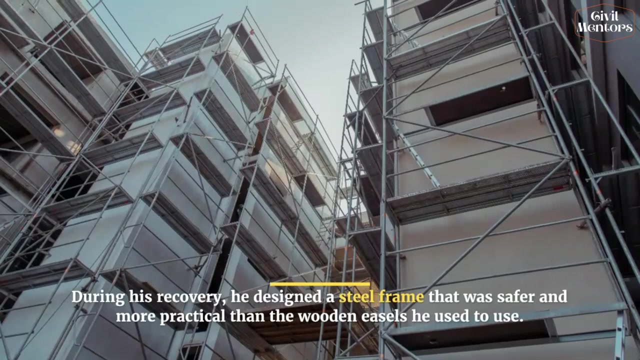 construction sites today. This system joined the tubular parts with clamps, screws and knots, achieving much more resistance and practical efficiency in the assembly. Another extremely important patent was the frame system created by a construction worker who had survived the fall from a collapsed wooden scaffold. During his recovery, he designed a 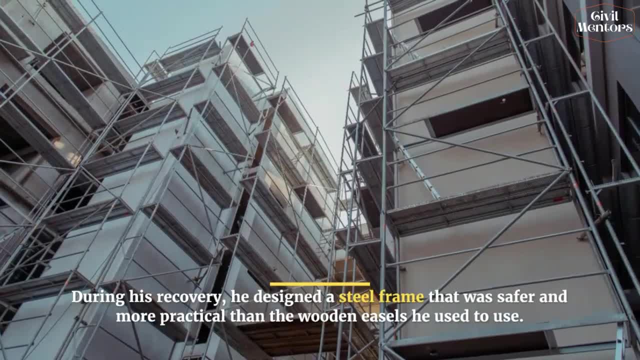 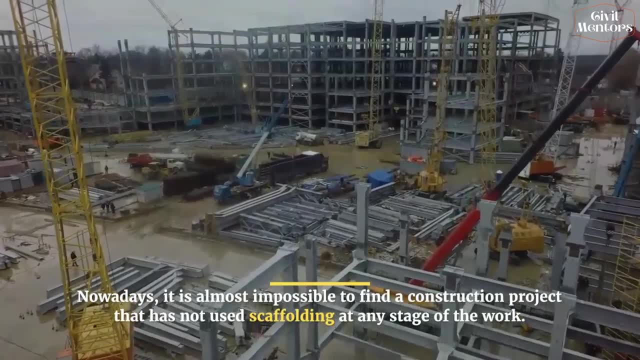 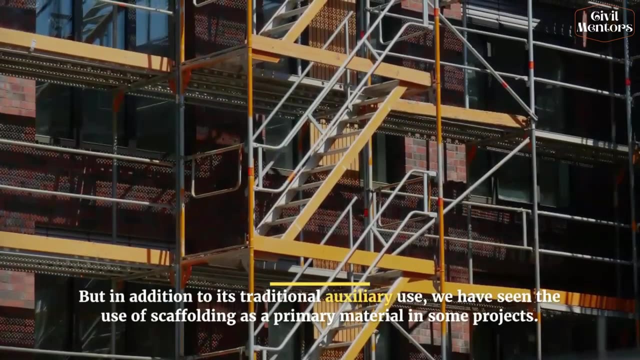 steel frame that was safer and more practical than the wooden easels he used to use. Nowadays, it is almost impossible to find a construction project that has not used scaffolding at any stage of the work But in addition to its traditional auxiliary use. 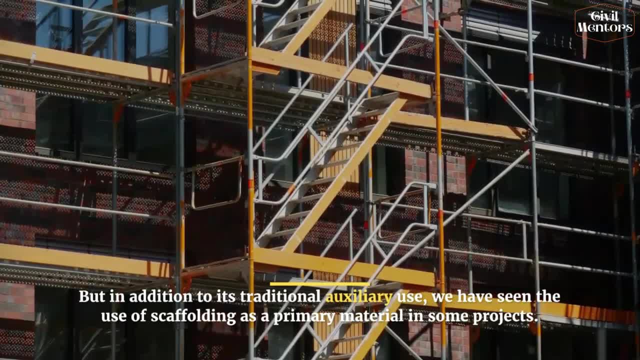 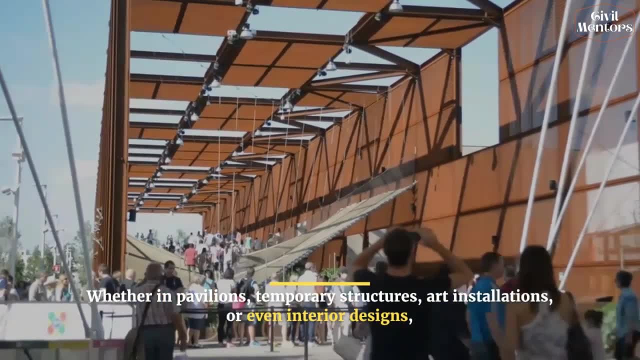 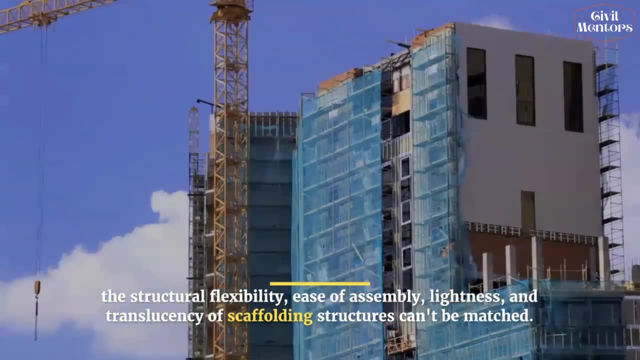 we have seen the use of scaffolding as a primary material in some projects, Whether in pavilions, temporary structures, art installations or even interior designs. the structural flexibility, ease of assembly, lightness and translucency of scaffolding structures can be matched.